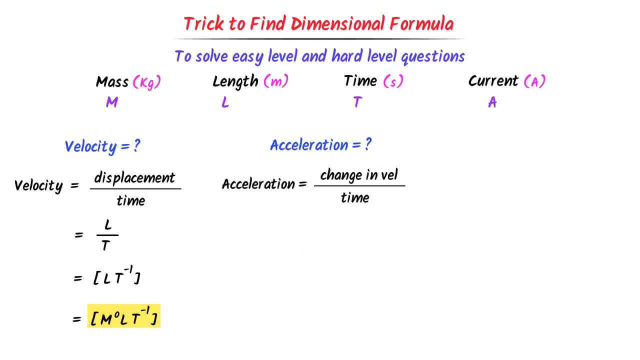 equal to change in velocity upon time. Now, velocity is equal to displacement upon time. Then, this time, We know that the dimensional symbol of displacement is l, that of time is t and that of time is also t. That information is equal to de существ de los 3.. It actually 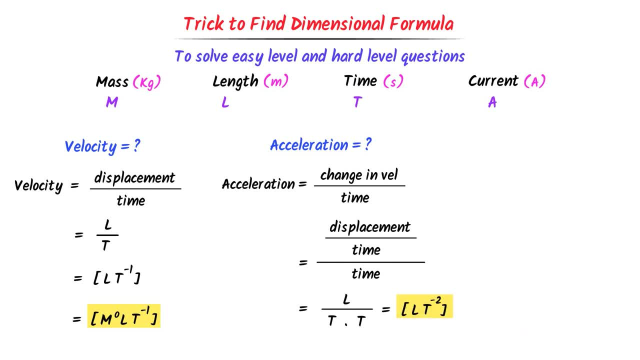 should not be understood. I do not think so. So I think, well, in this area, t to the power minus 2.. Hence, the dimensional formula of acceleration is l, t to the power negative 2.. Thirdly, find the dimensional formula of force. Well, we know that force, 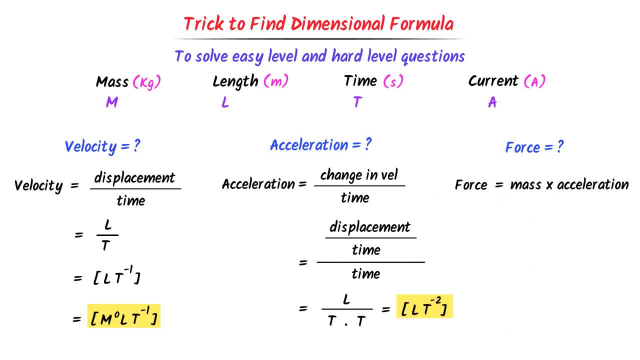 is equal to mass, into acceleration. The dimensional symbol of mass is m and we have already calculated the dimensional formula of acceleration, which is l, t to the power negative 2.. I get m l, t to the power negative 2.. Hence the dimensional formula of force is m l, t to the power negative. 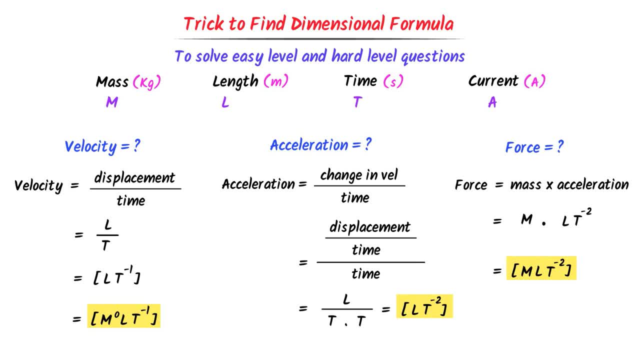 2. Note it down, all these dimensional formulas which I will directly use in hard level questions. Now consider these hard level questions. Find the dimensional formula of pressure, Pressure, stress and modulus of elasticity. Well, we know that pressure is equal to force. 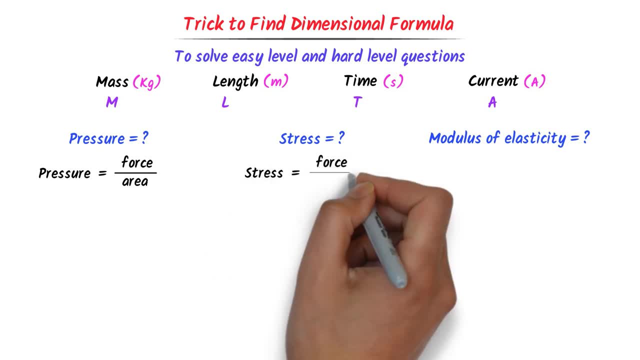 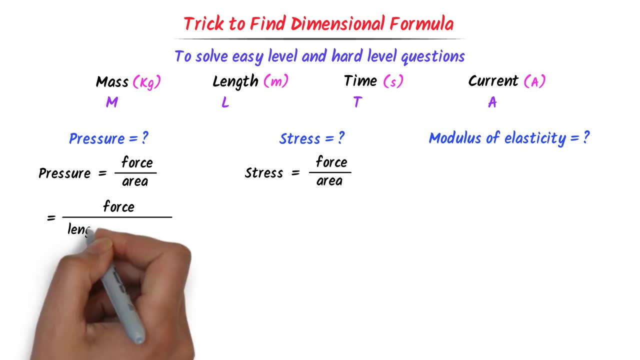 upon area and that of stress is force upon area. Now I write force upon. We know that area is equal to length and to breadth. We have already calculated the dimensional formula of force, which is m, l, t to the power negative 2.. The dimensional symbol of length and breadth is l and l. This l and this l squared, cancel. 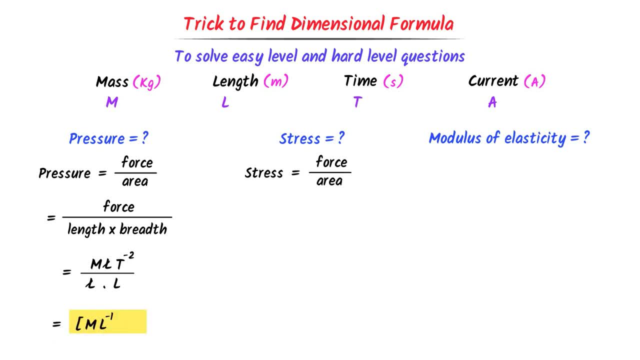 out, I get m l t to the power negative, 2 t to the power negative, 2.. Hence the dimensional formula of pressure and stress is square bracket: m l t to the power negative, 2 t to the power negative: 2, square bracket. 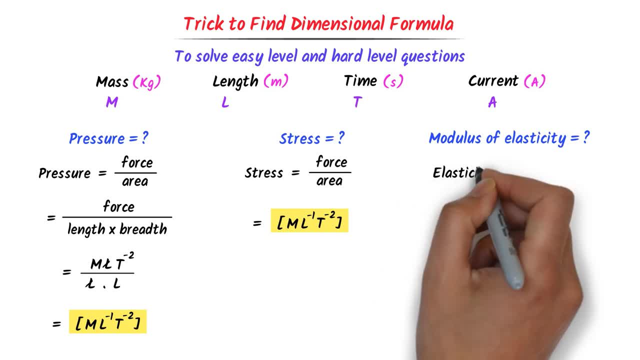 Meng Γιαoyi, PhD, MBA, JFK concentration A2. In case of modulus of elasticity, itsirosm夠 T sofortγз is equal to ε. Dean Вотagard, E Gmex Krisht Rostrom. Presentation Below. 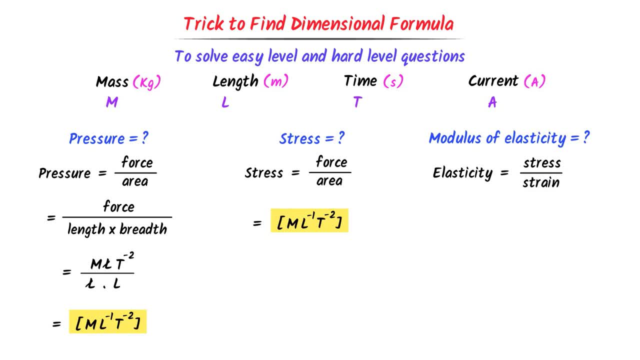 stress upon strain. We all know that strain is unitless. We get: modulus of elasticity is equal to stress. We have already calculated the dimensional formula of stress, which is M? L to the power negative, 1 T to the power negative, 2.. Hence, the dimensional formula of modulus of elasticity is M? L to the 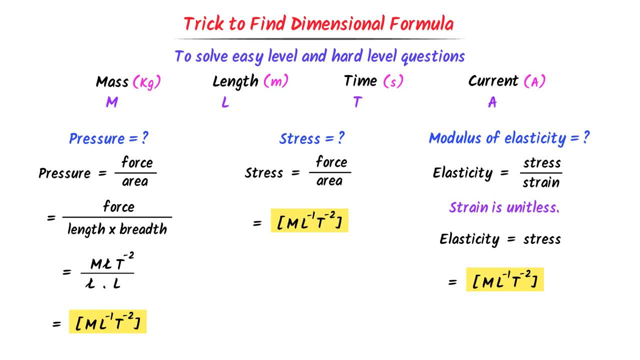 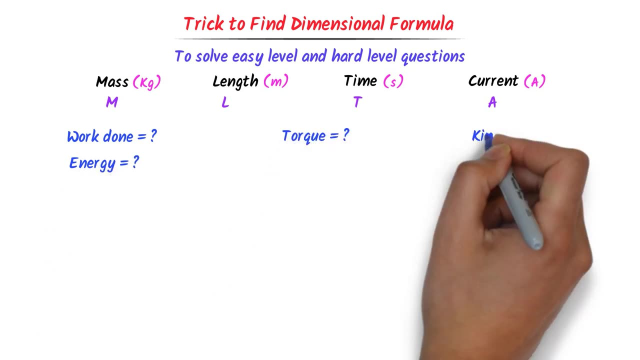 power negative 1, T to the power negative 2.. So these three physical quantities have the same dimensional formula. So note it down, all these dimensional formulas. Secondly, find the dimensional formula of Vorden energy, torque and kinetic energy. Well, Vorden and energy are the same, are two faces of the same. 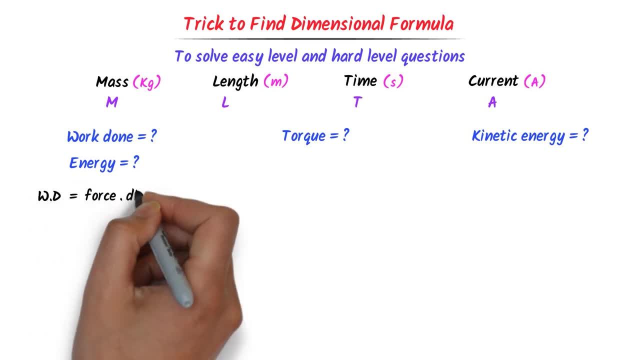 coin. We know that Vorden is equal to dot. product of force and distance. We have already calculated the dimensional formula of force, which is m, l, t to the power, negative 2, and the dimensional symbol of distance is l. I get m, l to the power, 2 t to the power. 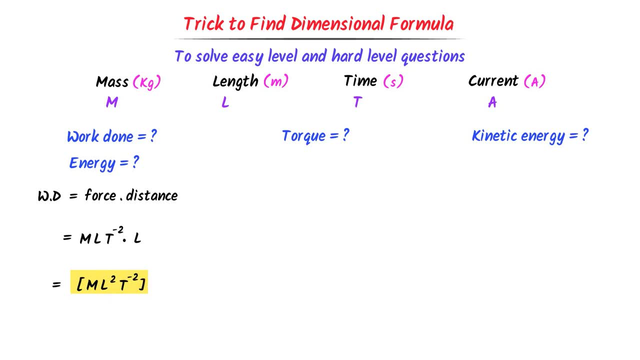 negative, 2.. Hence, the dimensional formula of burden and energy is square bracket m, l to the power, 2, t to the power negative, 2, square bracket closed. In case of torque, it is the cross product of force and distance. The dimensional formula of force is m? l, t to the power negative. 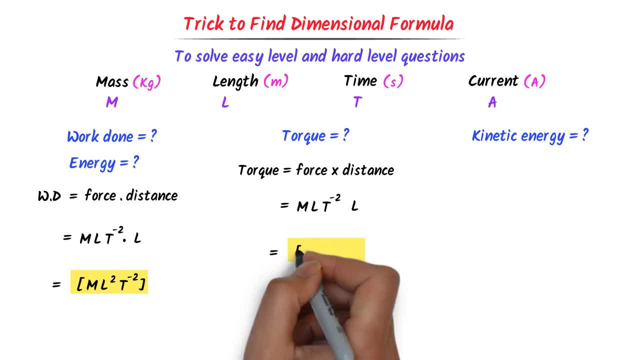 2 and that of distance is l. I get m? l squared t to the power negative 2.. Hence the dimensional formula of torque is m? l squared t to the power negative 2.. In case of kinetic energy energy, it is equal to half of mv squared. Remember that we do not consider constants. 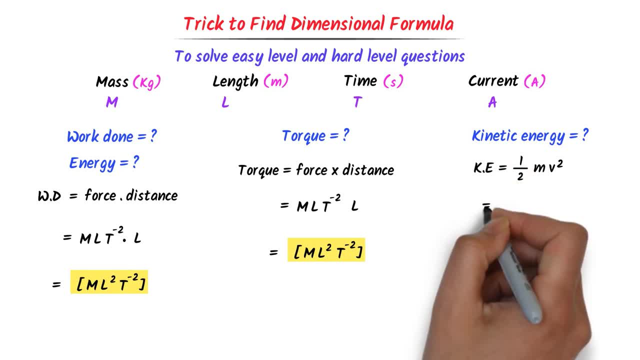 and dimensional formula. The dimensional symbol of mass is m and the dimensional formula of velocity is l? t to the power negative 1. I take square root on it. I get m? l squared, t to the power negative 2. Hence the dimensional formula of kinetic energy is also m? l squared. 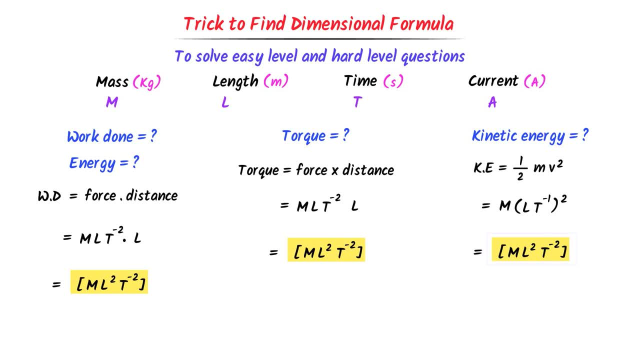 t to the power negative 2.. Thus, remember that the dimensional formula of all these quantities is the same, So note it down. Finally, find the dimensional formula of resistance, reactance and impedance. Well, according to Ohm's law, V is equal to I, R or R is equal. 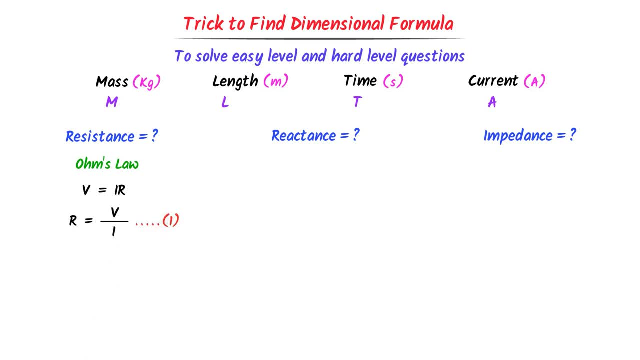 to V upon I Let. this is equation number 1.. We know that voltage is equal to mv squared 2 Varden upon charge. Also, we know that charge is equal to I upon time. So I write: V is equal to Varden upon charge. into time We already calculated the dimensional formula. 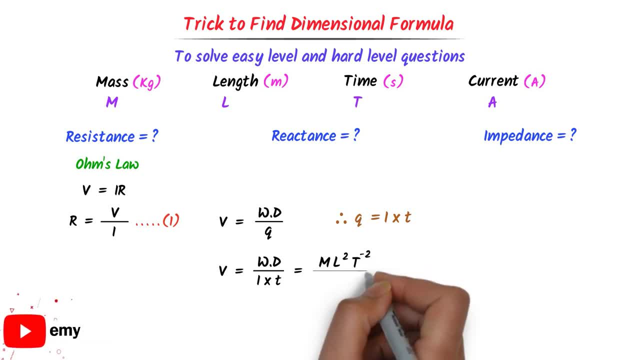 of Varden, which is m l squared t to the power negative 2.. The dimensional symbol of current I is a and that of time is t. I shift a t from the denominator to the numerator So that I get m? l squared t to the power negative 3 and 2 A to the power negative A. Hence, 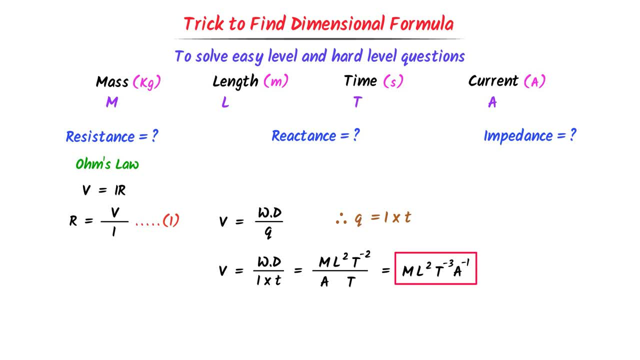 the dimensional formula of voltage is m? l squared t to the power negative, 3 A to the power negative 1.. Let, this is equation number 2.. Now I plug in this equation number 2 and equation number 1.. R is equal to the dimensional formula of voltage, is m l squared t to the 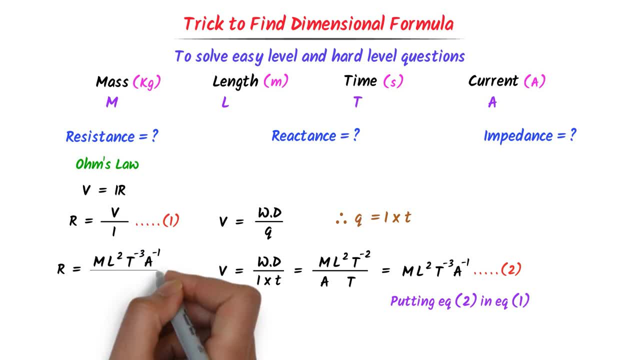 the power negative, 3 a to the power negative, 1 upon the dimensional symbol of current is a. I get mL squared t to the power negative, 3 a to the power negative, 2.. Hence the dimensional formula of resistance, reactance and impedance is mL squared t to the power negative, 3, a to the 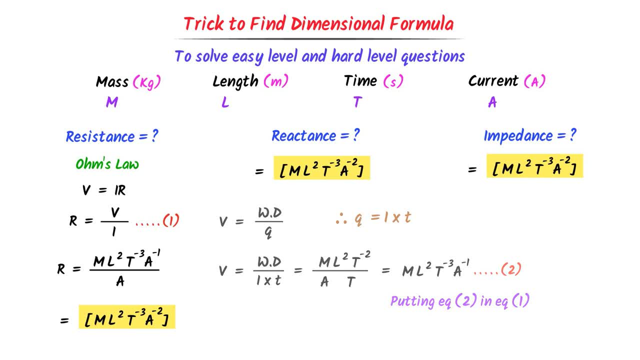 power negative 2.. Also, remember that the dimensional formula of Boltzmann, constant entropy and heat capacity is mL squared t to the power negative, 2 k to the power negative, 1. While dimensional formula of angular velocity, frequency and angular frequency is m to the power.